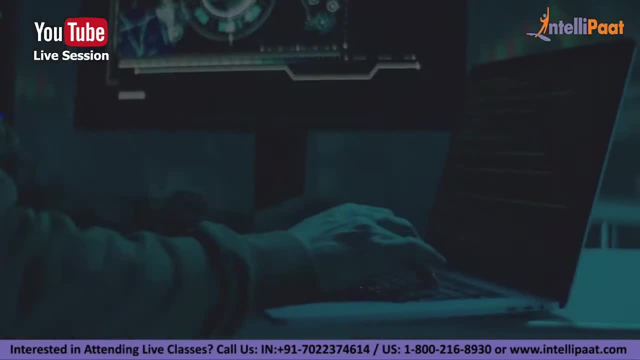 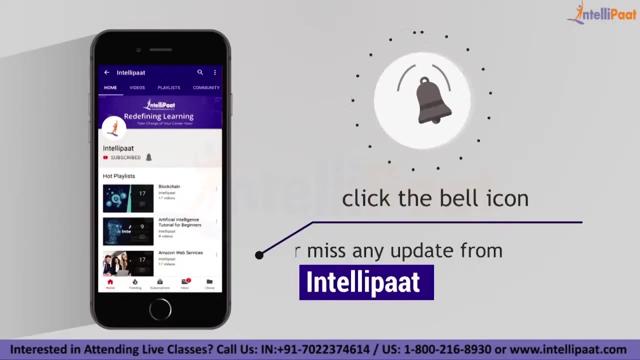 thoroughness and other performance parameters. In this session, you will learn all about software testing tools. Before we begin, don't forget to subscribe and press the bell icon to get latest updates from Intellipaat. Let's take a look at the agenda for this session. 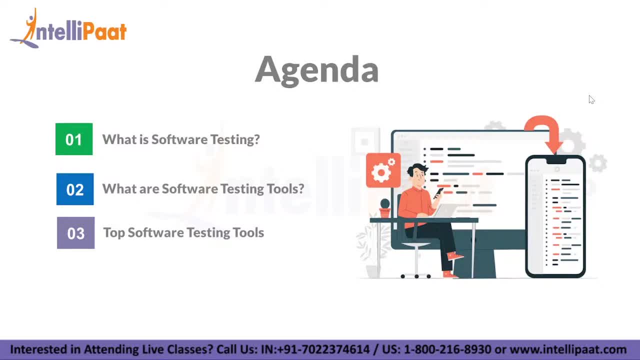 First of all, we will start with a basic introduction to software testing, And then we will discuss the importance of software testing tools. To sum up this session, we're going to discuss the various software testing tools at our disposal. I hope the agenda is clear to you. 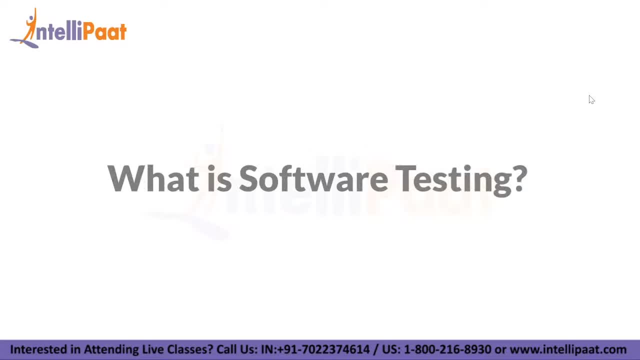 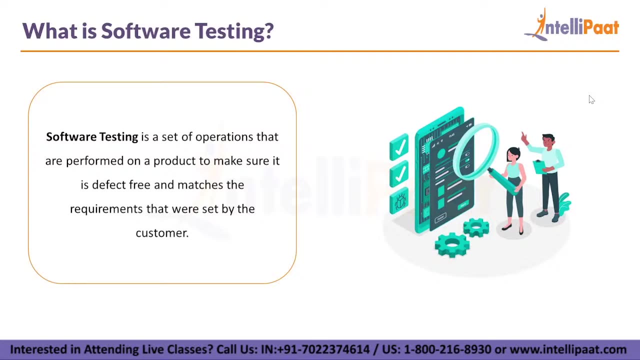 guys. So without any further ado, let's begin. What is software testing? Consider a scenario where a product releases without testing tools. The problems that may occur due to this can be disastrous. To start with, any sort of discrepancies will be met with expensive operations that will increase the cost of the overall. 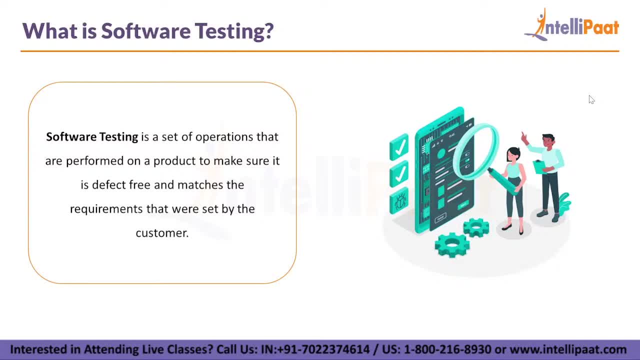 project. In simple terms, software testing is a set of operations that are performed on a product to make sure it is defect-free and matches the requirements that were set up by the customer. The various benefits of software testing include security, cost effectiveness. that, in turn, enhances the customer satisfaction. 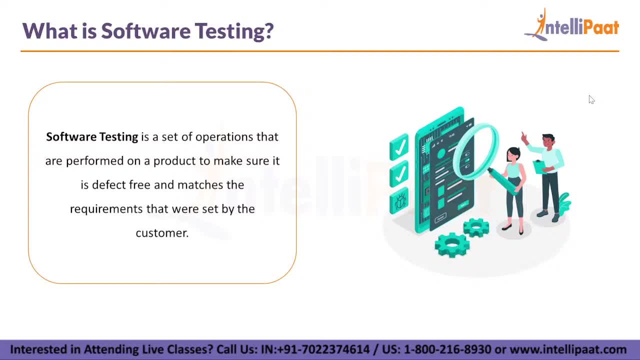 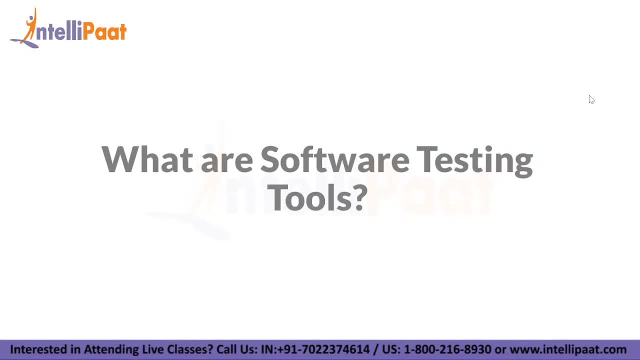 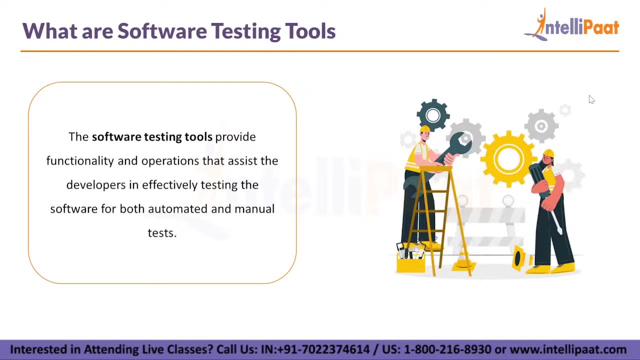 So, now that we have a basic idea of software testing, let's go ahead and understand what software testing tools are and why do we actually need them. So what exactly are software testing tools? Software testing tools provide functionality and operations that are going to assist the developers in effectively testing the software. 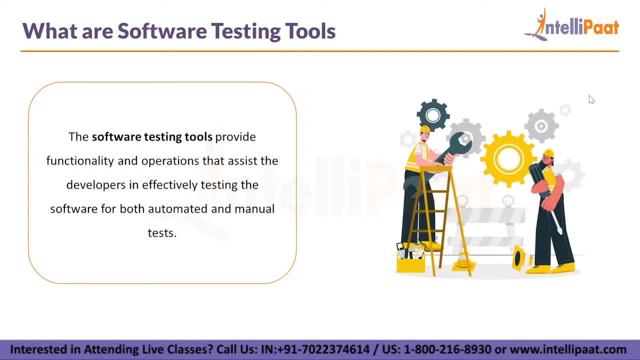 for both automated and manual tests. These tools will provide assistance in different areas where you will be able to perform automated tests: Software testing, cross-browser testing, mobile testing, security testing, and some tools even assist in test management, which can keep track of the progress in its entirety. 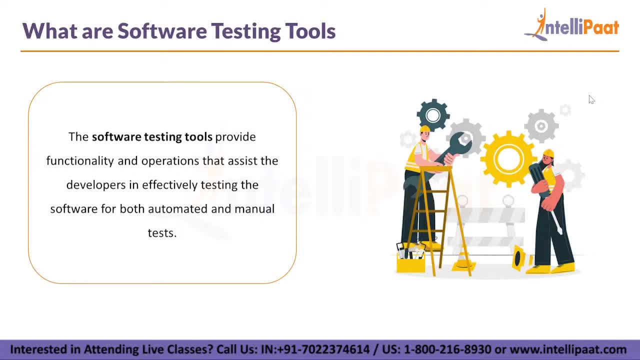 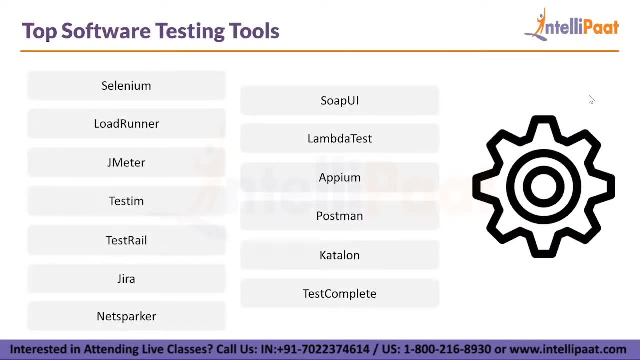 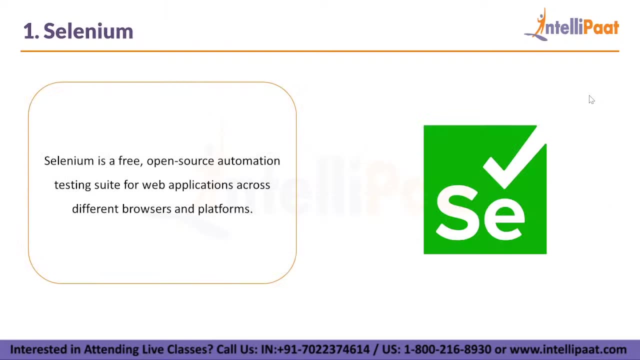 So now that we have a basic understanding of software testing and what the tools are, let's take a look at a few of the software testing tools. So we have curated a very short list of the software testing tools for you guys and we are going to discuss these in detail. First of all, we have Selenium. Selenium is a free 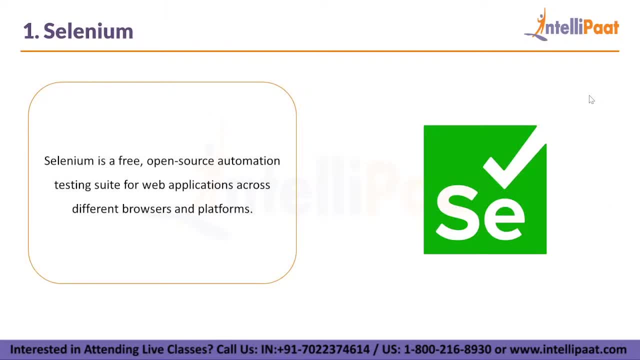 open-source automation testing suite For web applications across different browsers and platforms. Selenium focuses on automating web-based applications. Testing done using the Selenium tool is usually referred to as Selenium testing. Remember, only testing web applications is possible with Selenium. You cannot use it to test desktop applications or mobile applications. The advantages of 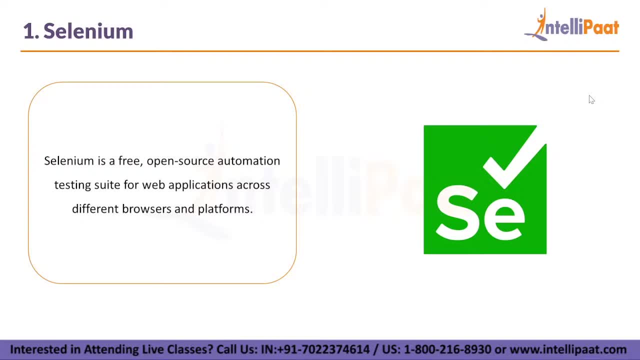 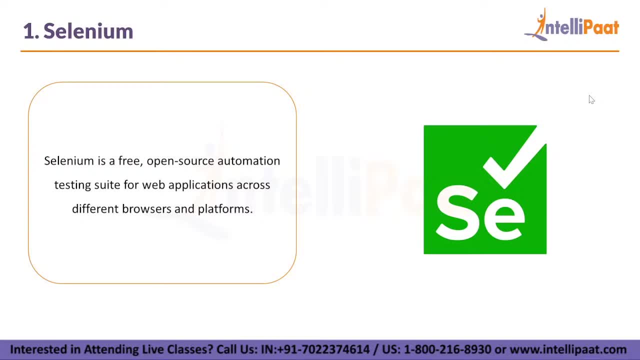 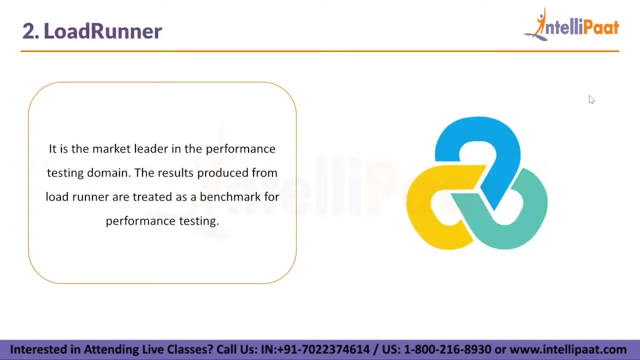 The testing through Selenium is supported across various browsers and operating systems as well. The easier implementation and ease of access makes it one of the most popular software testing tools. Now let's move on to the next tool that we have, which is Loadrunner. So it is the market. 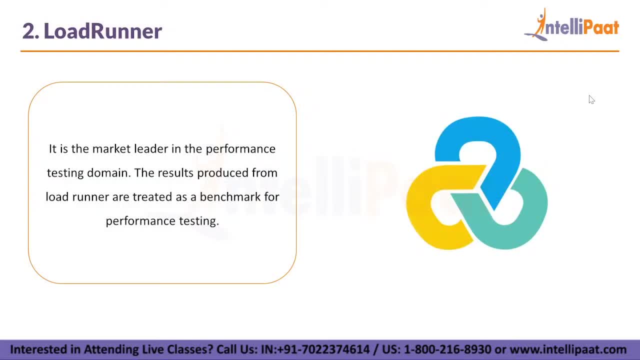 leader in the performance testing domain. The results produced from Loadrunner are treated as a benchmark for performance testing. The tool supports various development tools and communication protocols for performance testing. The results produced from Loadrunner are treated as a benchmark for performance testing. The tool supports various development tools and. 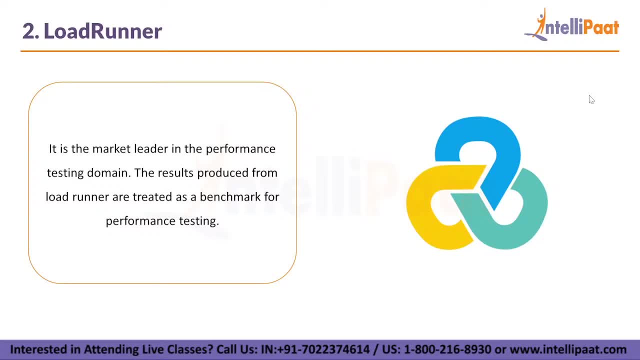 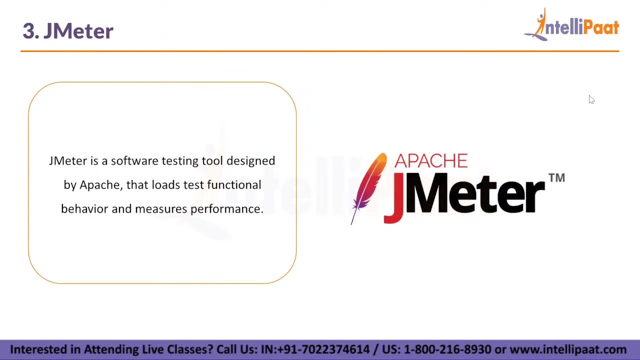 communication protocols for performance testing. The advantage of using Loadrunner is the reputation that it comes with. With over 80% market share, there is no other performance testing tool available that can match the Loadrunner. Next up, we have JMeter. JMeter is a software testing tool designed by Apache. JMeter loads. 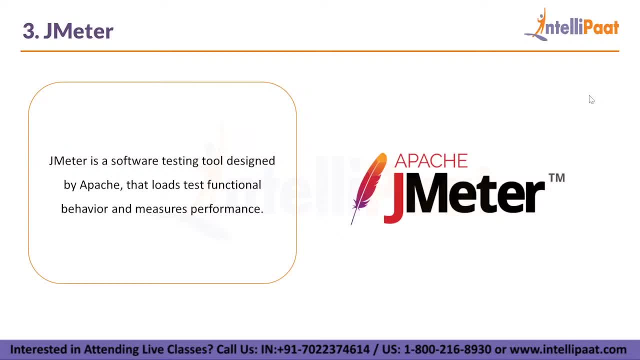 test functional behavior and measures performance. JMeter can be used for performance testing, unit testing or spike testing on various applications. The advantage of using JMeter is that it can be used for performance testing on various applications. JMeter is open source and provides 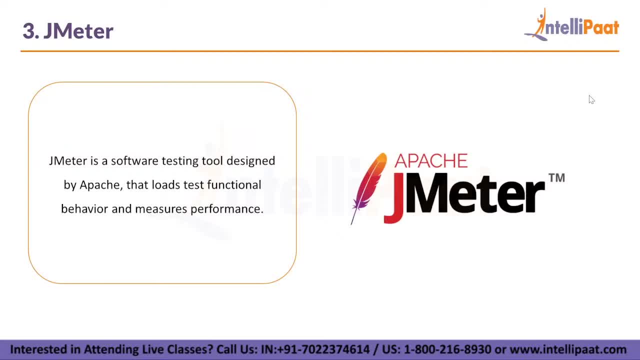 various browser plugins. It supports various tests and protocols with a GUI or graphical user interface that enables you to analyze test results in a variety of ways, including offline analysis. Next up, we have Test-IAM. The Test-IAM software testing tool is powered with artificial intelligence. You can use the AI-based software testing tool. 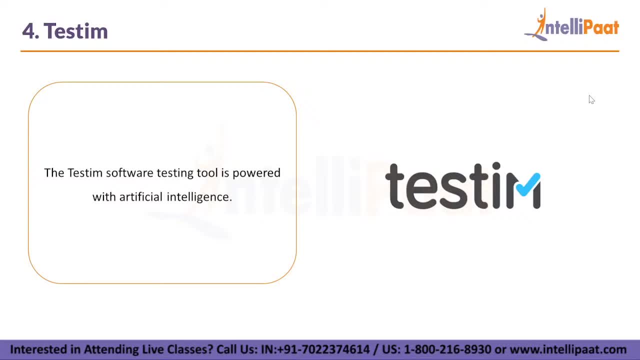 to automate functional tests. This tool speeds up the entire software testing process, The entire software testing process, through artificial intelligence. Next up, we have Test-Rail. This is a test case management tool that enables you to keep track of the entire testing process, with dashboards and metrics to measure the performance. The 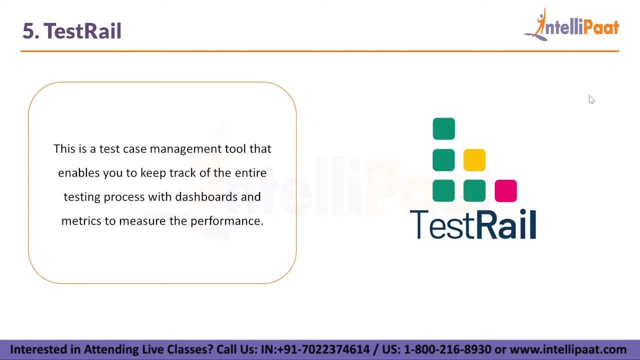 advantage of using a test case management tool is that you will be able to monitor each and every activity that will be involved in the entire testing lifecycle. It makes the job of the professionals very easy, and that's why it is one of the best testing tools for. 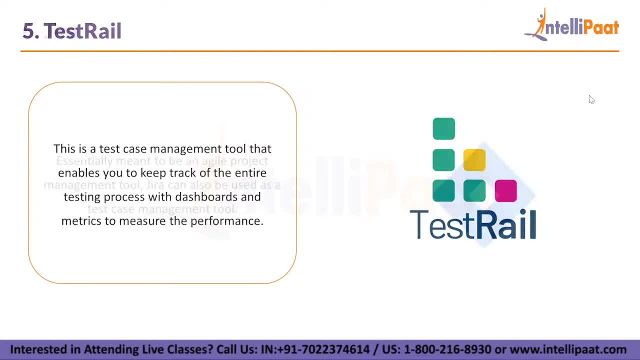 rès. Next up, we have Jira. Essentially meant to be an agile project management tool, Jira can also be used as a test case management tool. It keeps track of the defects and logging The advantage of being able to monitor the entire workflow for the software. 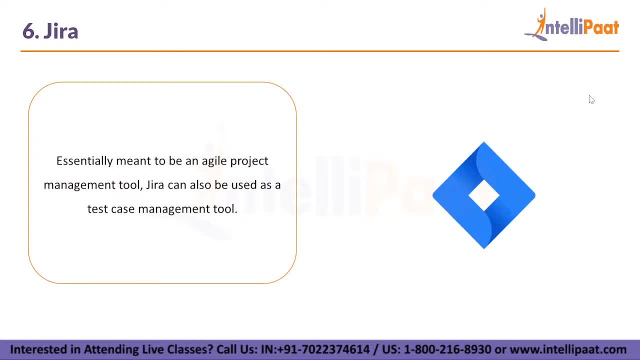 lifecycle makes Jira one of the most used test case management tools for software testing. Other Advantages include acceptance, functional integration, testing in Jira, along with the integration of various testing managers as well. Next up, we have NetSparker. The NetSparker is a 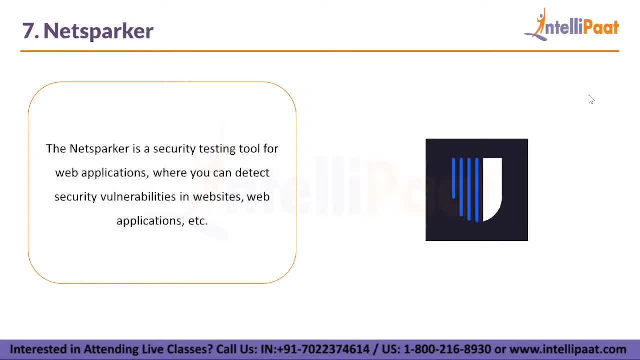 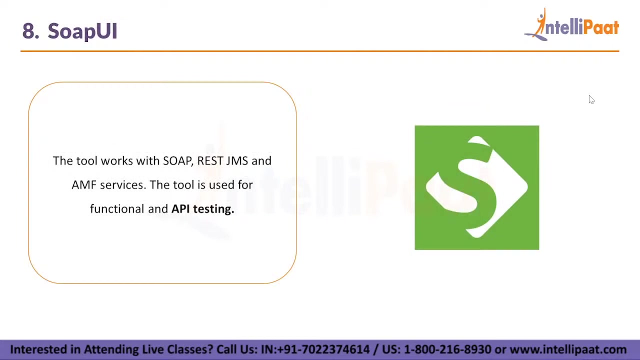 security testing tool for web applications, where you can detect security vulnerabilities in websites, web applications, etc. The tool is fully automated and the advantages include integration during the development cycle and is fully configurable with high efficiency. Next up, we have SOAP UI. The tool works with SOAP REST, JMS and AMF services. The tool is used for 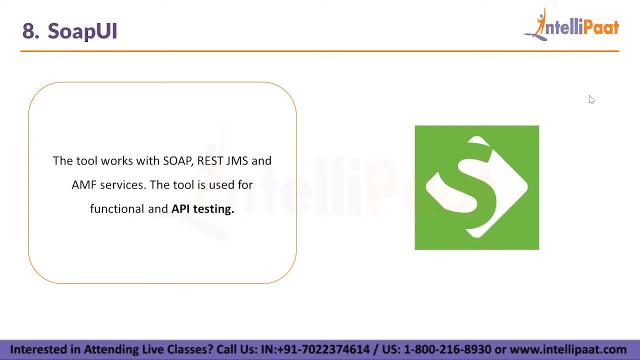 functional and API testing that also supports integration of SQL injection testing to identify security vulnerabilities. SOAP UI is the market leader in API testing and one of the most used software testing tools in the world. Next up, we have LambdaTest. LambdaTest is a cross-browser testing. 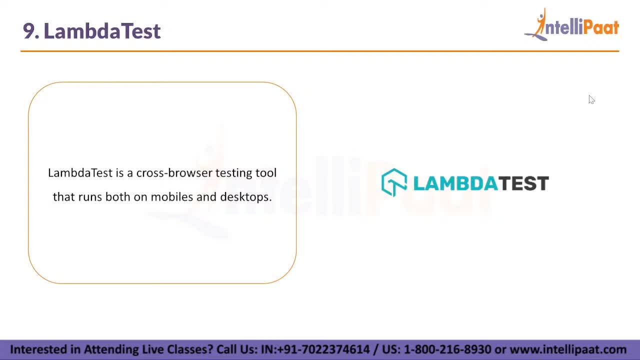 tool that runs both on mobiles and desktops. It can be used to perform test cases while, at the same time, efficiently perform live web browser testing. The other features included in LambdaTest lets the users test the whole website hosted locally. Responsive testing and debugging. support for the website is. 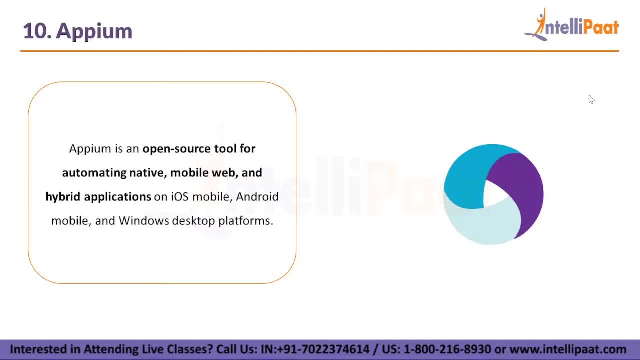 also included in LambdaTest. And, last but not the least, we have Appium. Appium is an open source tool for automating native mobile web and hybrid applications on iOS mobile, Android mobile and Windows desktop platforms. The various advantages of using Appium include that it supports both Android and iOS, where you can create the